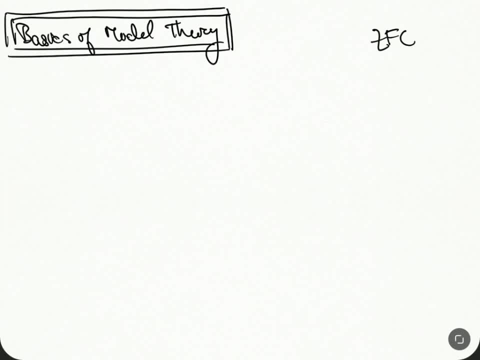 the semantic part and there's this syntactic part. Syntactic is this purely formal part where you kind of build up symbols and the rules for the symbols, And then the semantic part is where you try to assign meaning to these things. So so let me kind of give the basic idea. I'll just draw a little diagram here. So what we'll start with is we start with a signature. 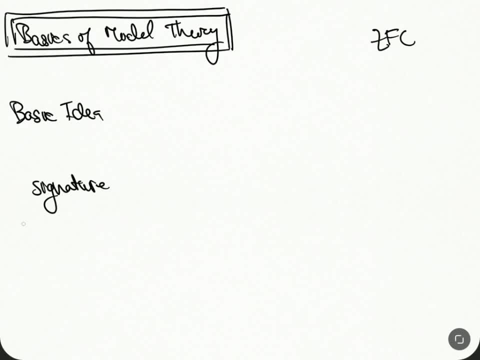 Okay, and what this is is just really something that encodes the symbols that you allow. So we're going to be doing things that are first order, that you allow. We're going to be doing things that are first order. So it could be like you know, you know these are going to be your functions, relations, you know constants, right, And this is going to be you know times. 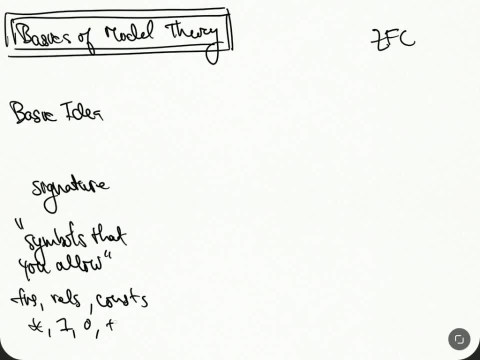 one, zero, maybe you know, plus things like this: Okay, From the signature, there are kind of two things that you can do. right, You are going to, you're going to develop structures, So these are semantic things, And then you're going to develop formulas, So these are more, these are. 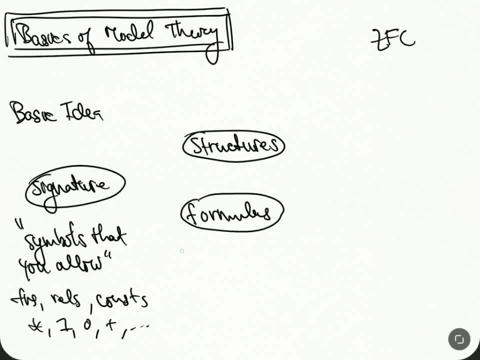 so these are syntactic again. So these are: this thing is things you can say, can say with symbols, And okay, so here in structures are So assignments of meaning to the symbols. Okay, if you hear that in the background, that's rain- I don't know if you can hear that or not, But there's a lot of rain going on. It's just like super miserable here, Okay, So. okay. so we have signature. from the signature we have structures and then we have formulas. So this is the language of formulas. 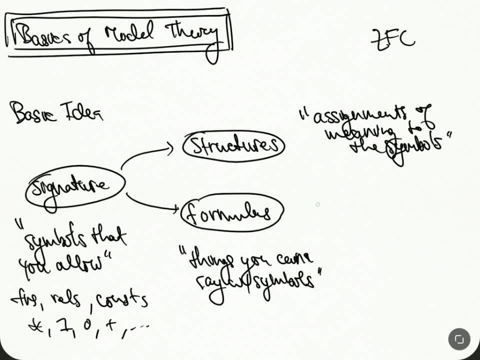 So to do this, you have to build up these things called terms. we'll see this, And then, inside the formulas, you can take a subset of formulas, And these are theories, Okay, And so these are a set of like axioms that you could have. Okay, That being said, let's just kind of move forward, And we'll do. we'll do signatures first. 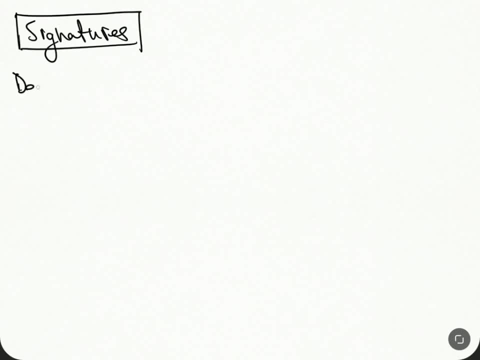 Okay, So let's define a signature. So a signature is a tuple Sigma consisting of constant symbols of the signature function, symbols of the signature relation, symbols of the signature function. So then there's this arity function. There's two kinds of functions. 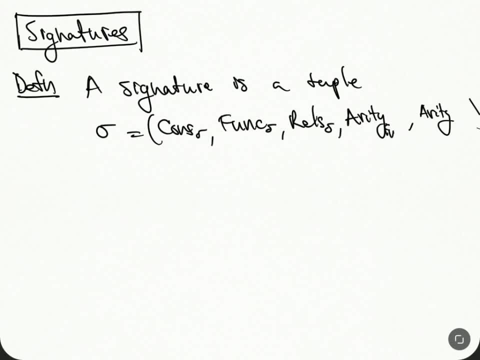 one for the relations symbols and one for the function symbols. Okay, so this is going to be a mouthful, So I'm just going to do this as so this will be C, sigma, F, Sigma, R, Sigma. Okay, and then I'm just going to call both of these guys. 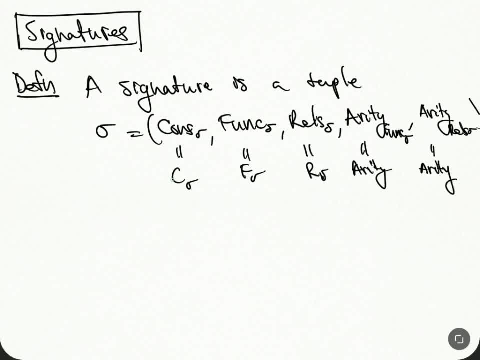 arity. okay, these are all sets. so C, Sigma, F, Sigma, R, Sigma are an element of sets. okay, and then arity, so it's a. my voice just cracked, that's okay. so the arity for the function symbols is a map from the function symbols to the natural numbers. so this tells you how many inputs it can have. or you should think. 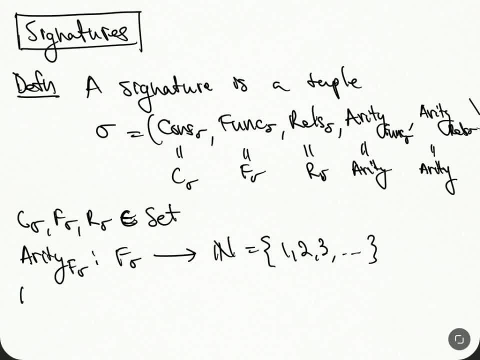 of it that way. really, it's just a function. it has no meaning to it right now. so right now it's like we're making random stuff without any meaning to it, but it will have meaning. so my natural numbers are going to include one. I'm going to do this American thing, okay? so this is what a signature is. a signature. 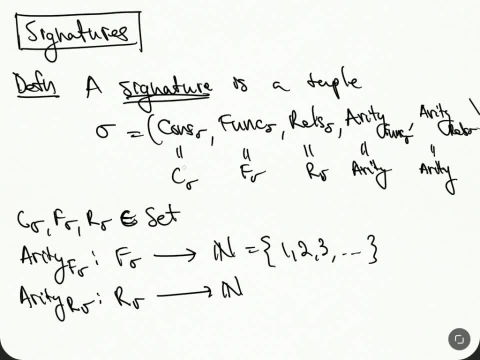 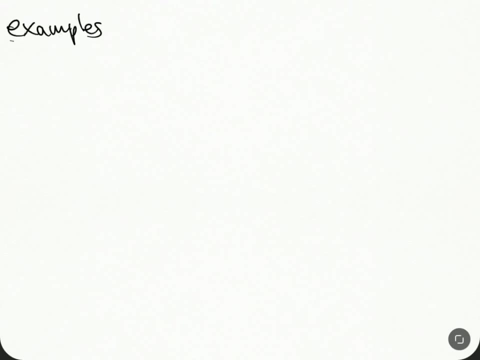 is this blah, this, this syntactic, black right, it consists of some sets and some functions. what we're going to do is is we're going to build. so when we do theories right, when we talk about familiar structures, we're going to have signatures associated to them. so let's just give some examples real quick. so, the signature for rings. 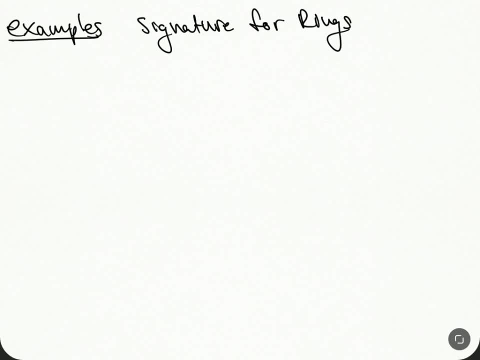 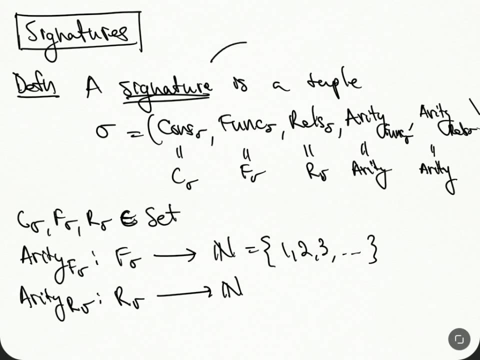 okay, let me say something before we go back here. so this is um, this is one sorted, so this is single, this is what's so called single sorted. so sometimes your signature is going to have constant, like a bunch of these, so you're gonna have multiple sorts. so like 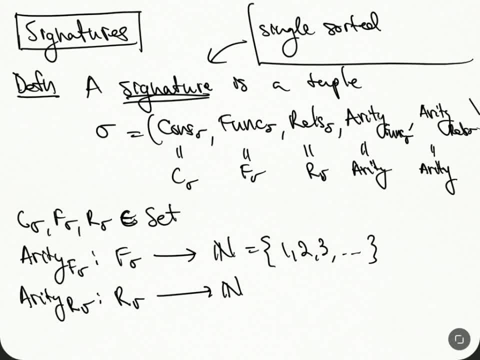 a sort. a sort is. a is another set where you can do this and sometimes you encode it in multiple sets. a good examples of this is valued fields. so in valued fields you have kind of a residue field sort and you have a, the value group. so sometimes you want to include. you know, you don't just want to talk about the- 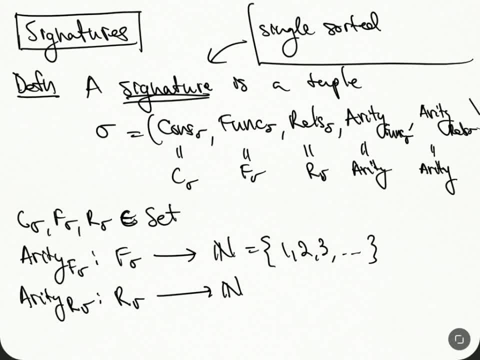 field. but you want to talk about the residue field and you want to talk about the value group. well, these, the, the residue field and the value group, aren't the members of the sick, aren't same members of the field? so sometimes you need to add extra function symbols, so like, so like, let me, let me, let's talk. 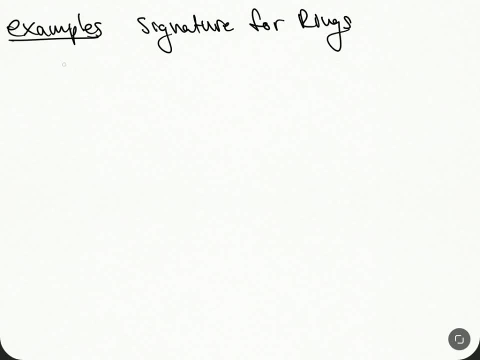 about this for a second. so in the signature for rings. so the constant symbols I'm just going to do is C and omit the sub Sigma. we're going to have zero and one F is going to be plus times and then we're going to have this minus. 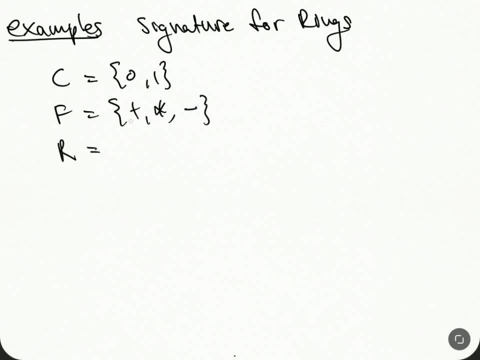 symbol, and then the relation symbol is going to be the empty set, So there's going to be none of them. And then the arity for each of these, the arity for the function symbol here, plus times the arity for minus. So this is 1,. 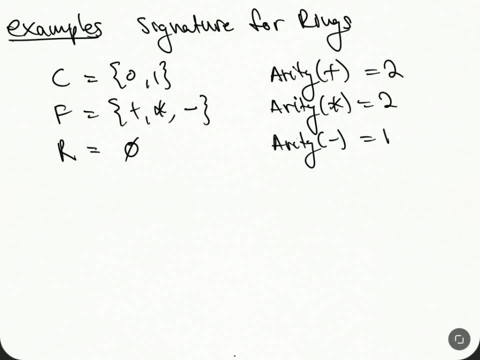 this is 2,, this is 2.. Okay, so here's the signature for rings. We have just two constant symbols: we have these function symbols and then we have these relation symbols In the first order formula. so these are things like: 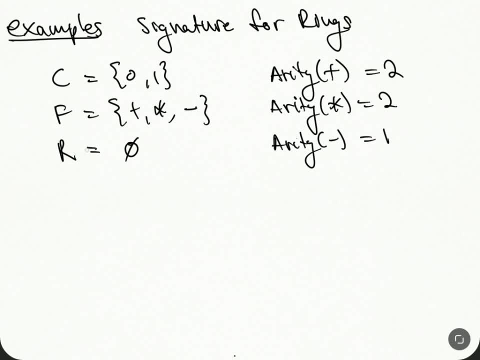 for all x and y and blah, blah, blah. we're going to be built out of these symbols. Okay, So if we wanted to make them, ordered rings. so how do I do this? Let me make a color. Oh, there we go. If I wanted to do. 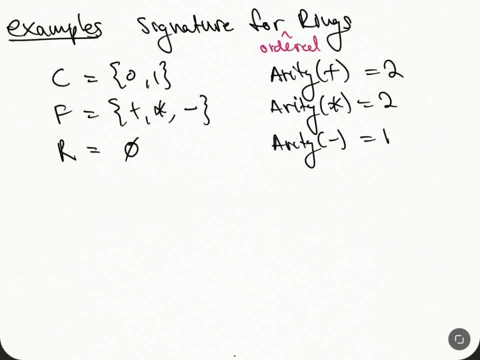 ordered rings, so we would get rid of this here. then we would do: the relation symbol would be this one instead. Okay, So if we wanted to do ordered rings, so we could have a ring with an ordering, Okay Again, I haven't. 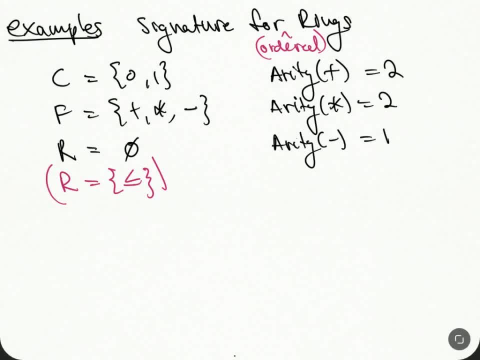 really assigned. I haven't said this is a ring. I haven't said that they satisfy axioms. These are just the symbols. you need to talk about rings. There's much simpler examples. They don't need to be so complicated. So, for example, you could just do groups. 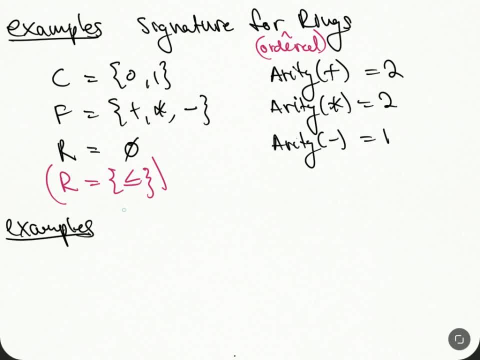 or you could just do graphs, So for example, for the signature, for graphs, for graphs, Okay, Let's do this. Okay, Here you're just going to have no constant symbols, You're going to have no function symbols, And then. so I'm thinking of graphs as just 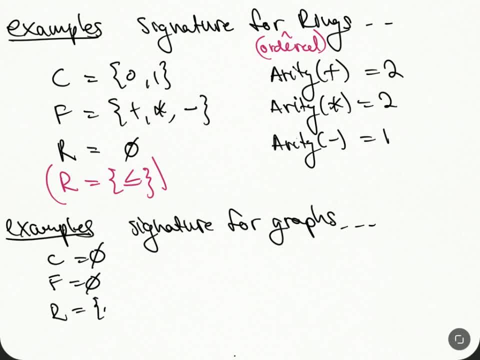 being encoded by the vertices. So here there's just going to be a single edge relation. So this will be the incidence relation, Okay, Okay, And we'll be thinking of it as taking values on the edges. So the arity is just going to be 2.. 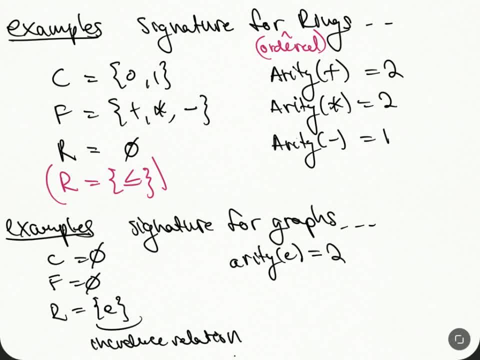 So yeah, I'm sorry, It's just going to take values on the vertices. So you plug two vertices into this thing and then it's going to give a thumbs up or thumbs down, depending on whether or not it's true. I mean that's. 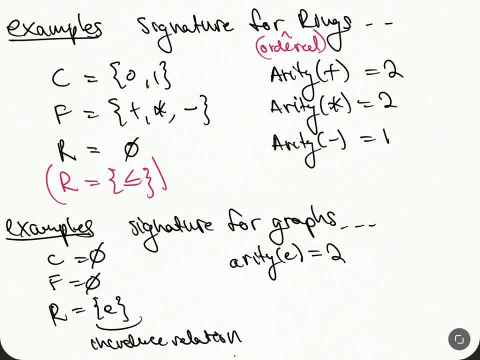 in the structure, But right now it's just the symbols. Okay, So we're assigning no meaning to them. Note here that I've only included the vertices for the graphs. There could be a version where I had a multi-sorted version. 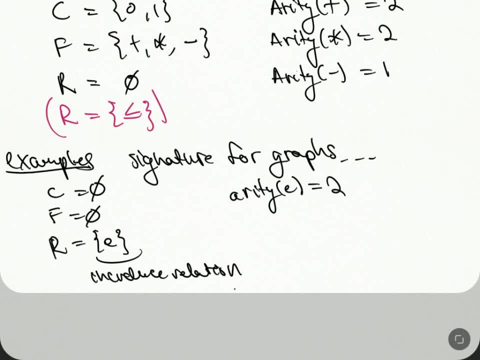 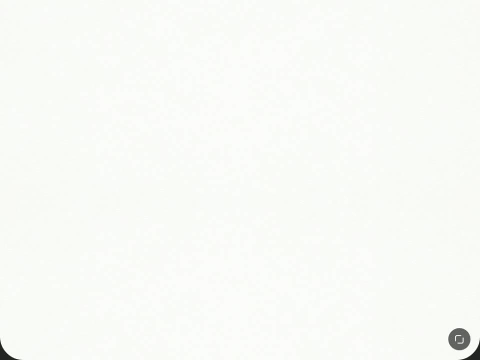 where there was something for the vertices and for the edges, But we'll not talk about this in this video. Okay, So I said that we had this signature And now we need to talk about formulas. Okay, So, So languages, So formulas. 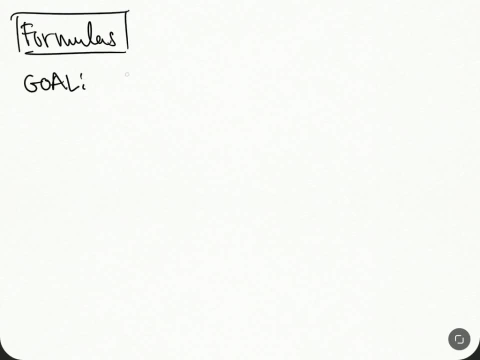 So our goal is to build a set of strings- L-sigma- So these are going to be the formulas. So the first order for a signature. Okay, So these are going to be the formulas that we can talk about Again. this is all syntactic, Okay. 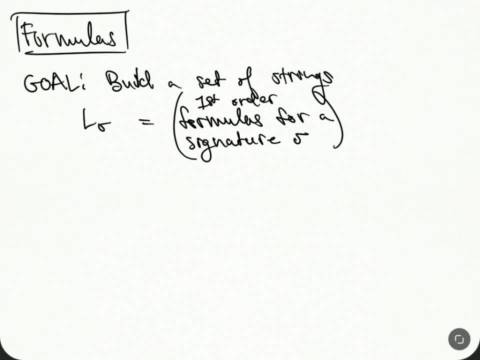 So this thing is going to be built up inductively. So this is the idea is to build this idea, Build Up these strings, Strings, inductively From so-called terms. So this would be T-sigma And okay, and then the idea to build the terms: 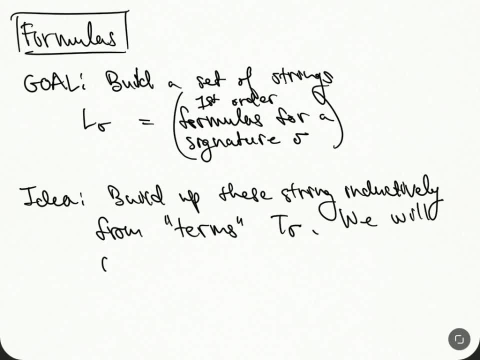 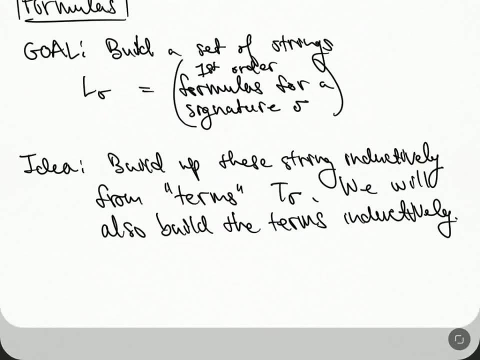 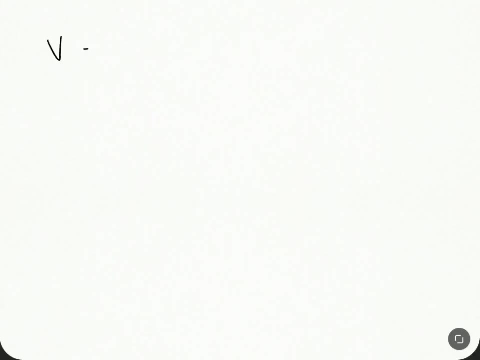 We will also build, Build, Build The terms inductively Okay. So to do this we first need a set of variable symbols. So V is going to be a set of variable symbols. So I guess the language here. I wrote L-sigma here. 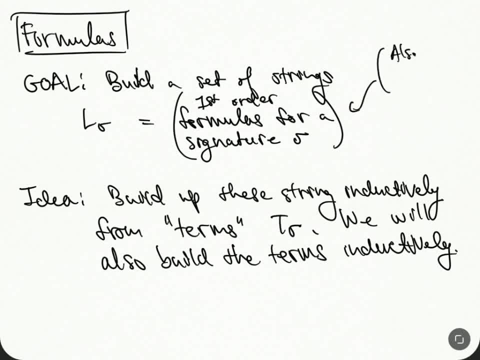 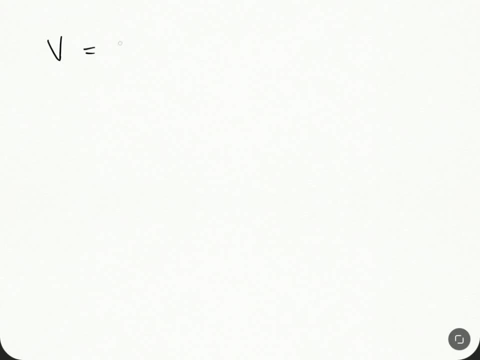 This also depends on the variable symbols. Okay, That's not too important, So this is just going to be a set Of variable symbols. So right now I'm starting the construction. So this is a set, Just a set, Okay. 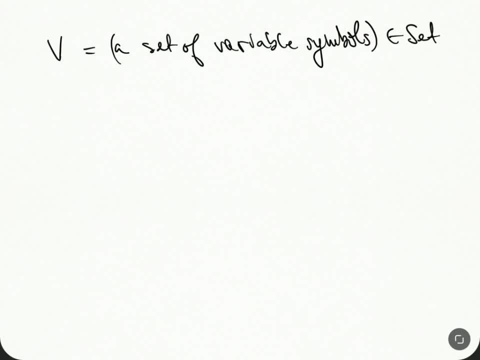 Terms, Okay. So now I said that we're going to do terms, So there's kind of like a little subsection here, So the construction of terms, Construction. Then we're going to use the term of T-sigma, Okay, First of all, there's kind of going to be a base case. 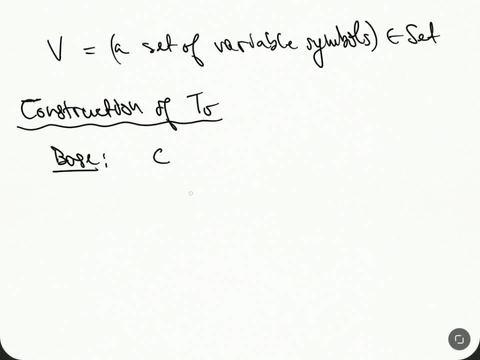 Okay, The base case says that C- these are the constant symbols- are going to be contained in T-sigma, So we're going to throw those in And then we're going to throw the variable symbols in. Okay, So we have constant symbols. 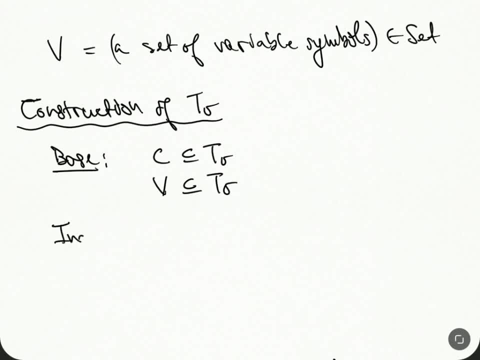 We have variable symbols, Okay. And then there's this inductive step Which says the following: It says that so for all functions. so if okay, so if let's say f is a function, okay, and 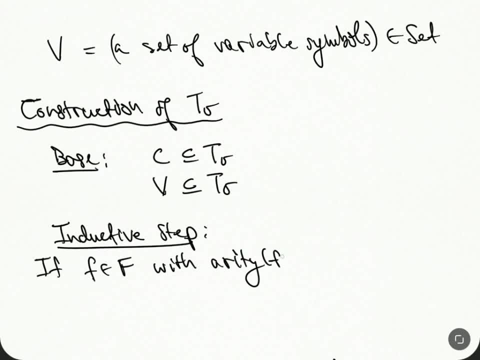 with arity n and if we have some terms already. so if T1 through Tn are already terms, then we're going to say we're going to throw this new guy in here, We're going to throw this new term in here. 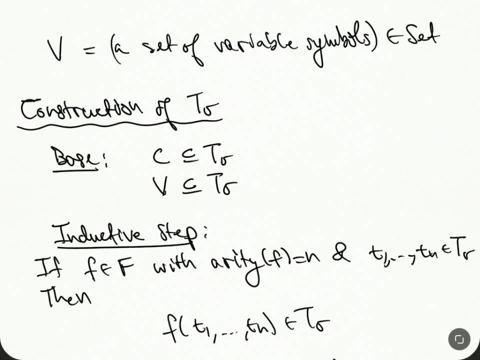 So by making a new thing, So like in our, in our ring case, we had two terms, We could add two terms, Okay. Okay, So we, this is the construction of T-sigma. So we have the constants, we have the variable symbols. 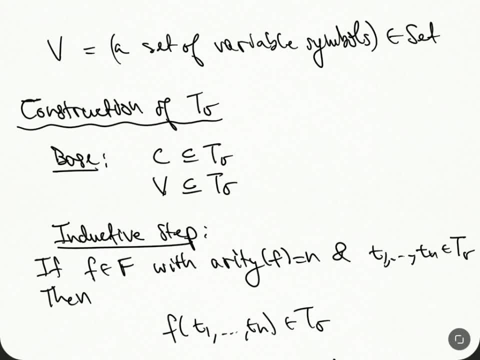 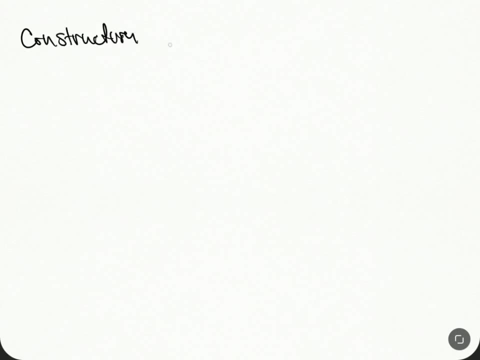 and then we build them up by, by kind of composing terms. These functions, So like iterating our, our functions. Okay, So now we're going to be talking about the construction of the formulas. Formulas, Then I did it with squiggly. 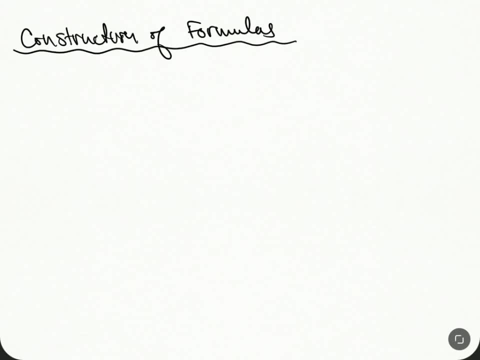 Okay, So we're going to talk about the constructions of formulas. So again, this is a two-step procedure In the base case, right, Okay? So the base case says that. so for all two. so there's kind of two things. 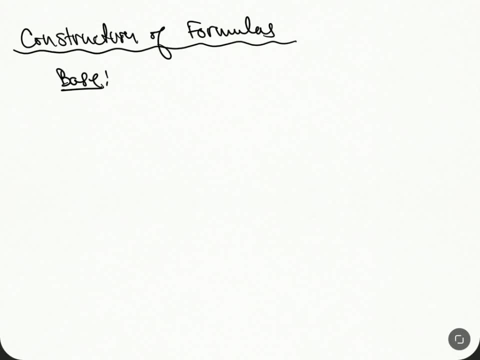 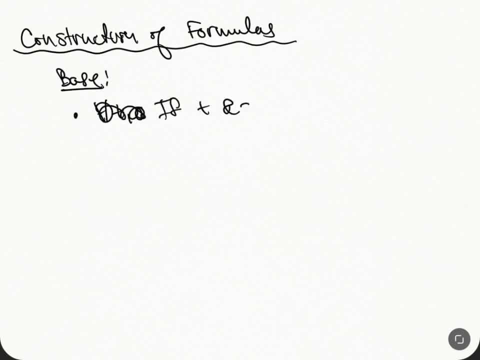 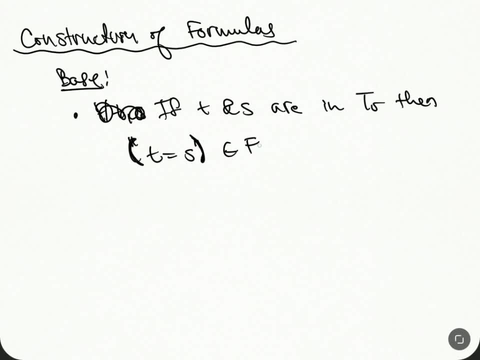 so, so. so formulas okay. so the next base case says that for all relations up, sorry, let's do it the same kind of notation. if R is a relation in the area of R, let's say with kind of a bad one, huh, oh, okay with, the area of R is equal to N, and let's say T. 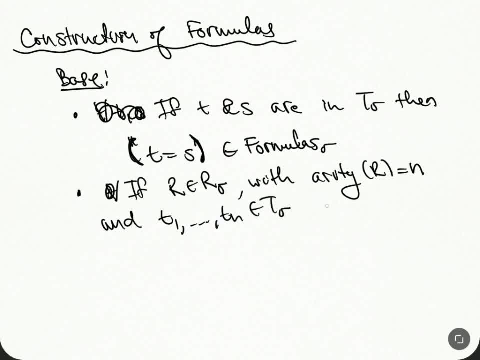 1, T, n are terms, then the formula will do with parentheses R, T, 1, T, n. so this is this, just the string. so when I do these parentheses here, I'm just meaning the string. so this is in formulas okay and so okay. so now, now we have these, these kind of 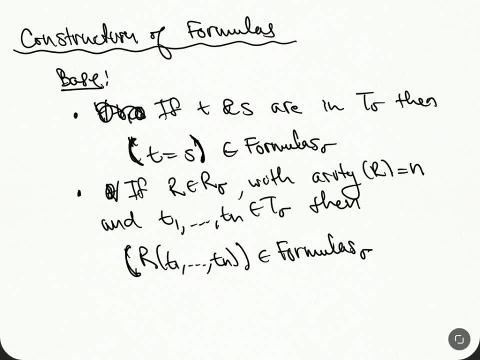 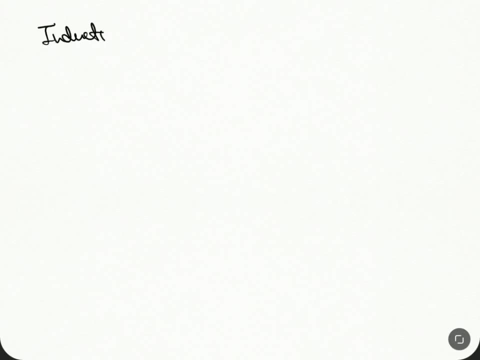 base formulas, and now I'm going to talk about the inductive step. so, the inductive step: I guess I need a new, new page, okay, so okay, what's the first thing says? it says: if P and Q are formulas, so this is this means they're in formulas of Sigma. 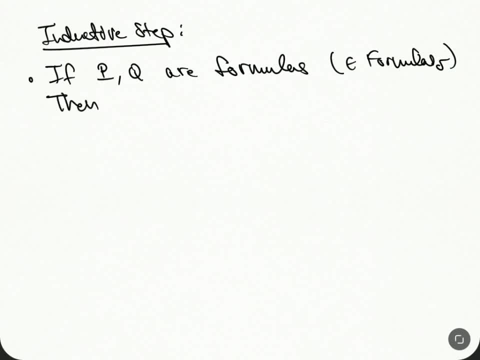 then you need to do this. if you're going to be using Lewis river, so you're going to use a new N, and if you you're going to do n of sigma, then you're going to use N of sigma, then you're going to. Then the following will be formulas: 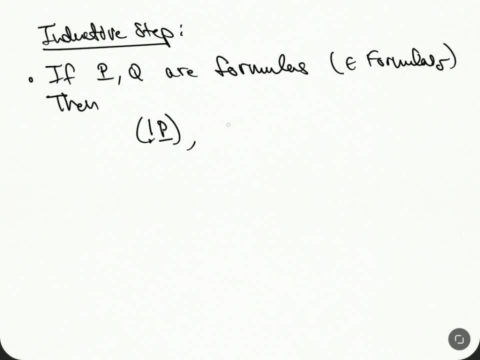 Not P, P and Q, And P or Q will be in formulas. Okay, So to continue, right now I need a definition. So, as we've constructed the formulas, right now a formula here will look like will depend on some number of variable symbols. 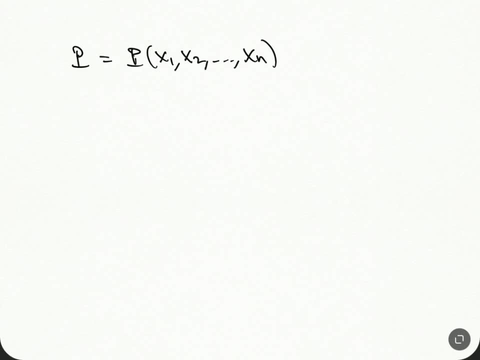 So formulas depending on. so this is notation for a formula depending on variable symbols, And what we can do is these are called free variables here, Free variables, And what one can do is one can bound them. Okay, So the free variables are the ones that are not going to be. 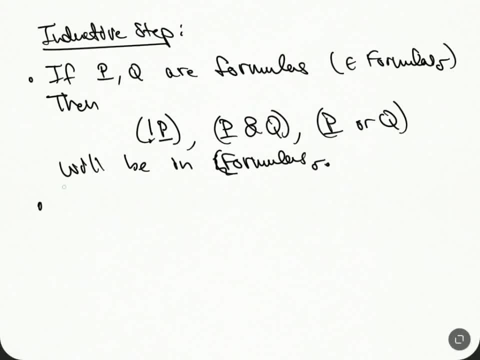 quantified. Okay. So for any formula, the formula for a fluid in a particular formula is the one that we set aside to get a fundament. okay, The value of the animation of a 100 end prong: Okay, Okay, we'll be included. 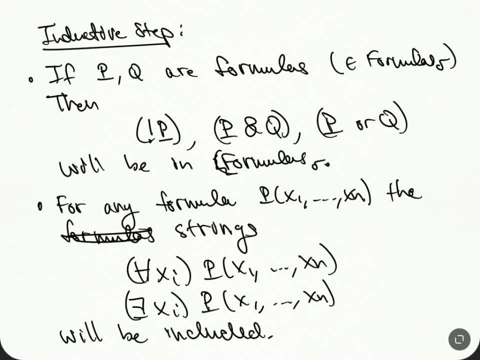 Okay, and so these things need to be free variables. So, after this process, they become bounded. So, after this quantification process, these guys here become bounded. Okay, so these are bounded, All right, So these are bounded. So these are bounded. 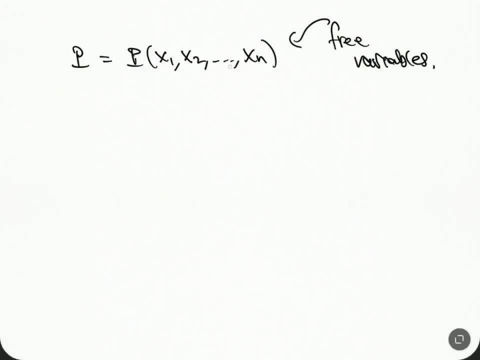 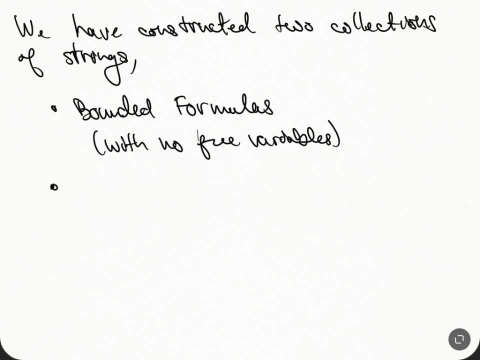 They become bounded variables. Okay, so these are the free variables. like I said, We've constructed two collections of strings, Okay, the first one So the bounded formulas, So these are with no free variables. And then we've constructed formulas which have free variables. 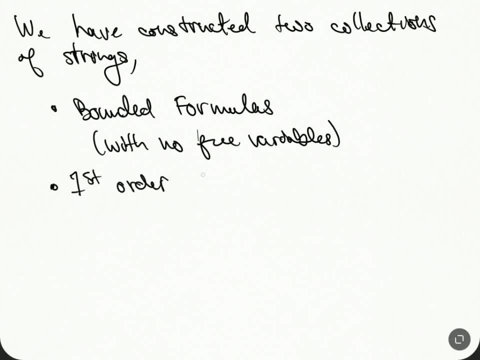 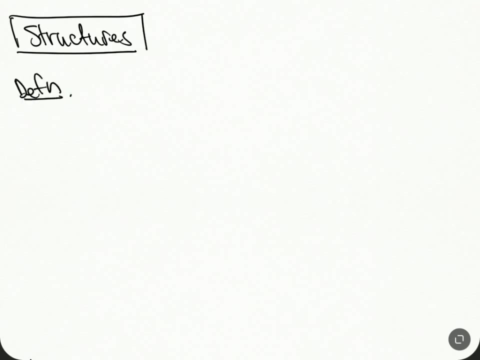 First order formulas. So we've constructed them with free variables, free variables, free variables with free variables. So we're now going to talk about structures, matrices, soupocking with So definition. So let sigma be a signature. So in a sigma, structure is a tuple M, C, R, F, where M is a set. 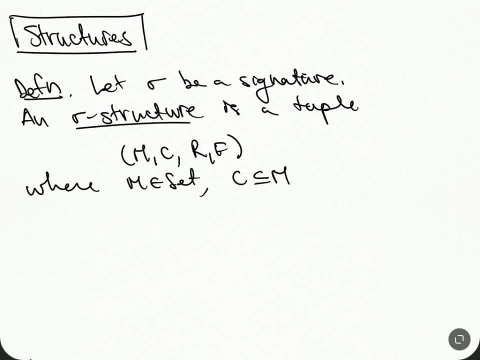 C is a subset of M. C is a subset of M. C is a subset of M. C is a subset of constants. Okay so C is a constant and R is a set of relations on M and F is a set of functions on M. 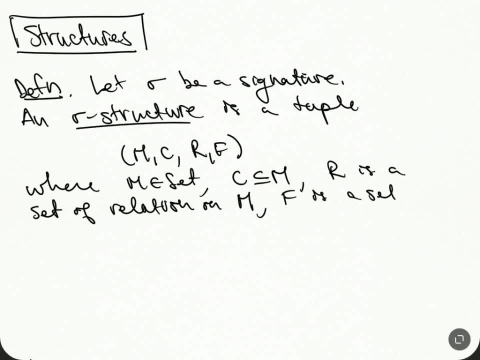 C is a subset of M. C is a subset of constants. Okay, that respect the arities. Okay, so what it is is it's an actual set of constants, relations and functions. Okay, and then they're going to. 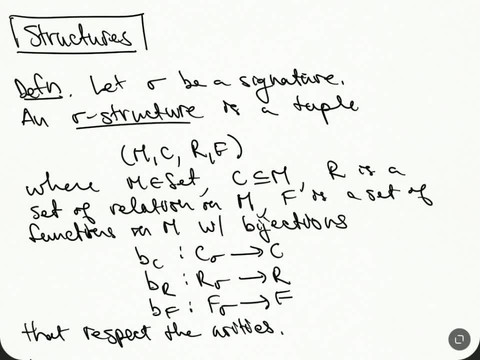 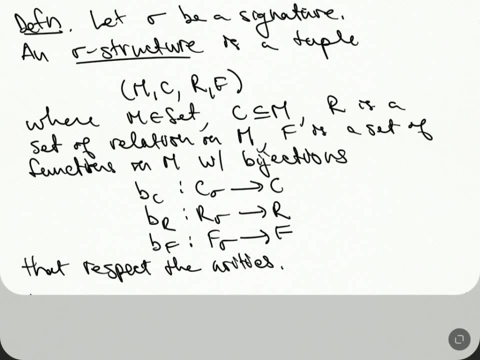 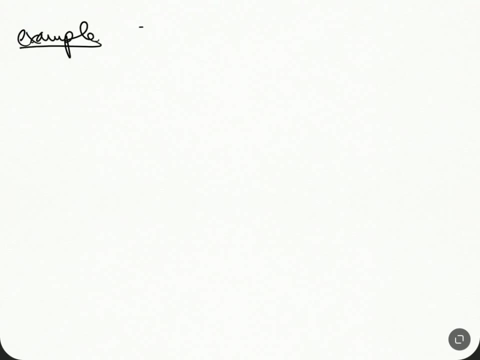 match the signatures, okay. So it's pretty stupid. to be honest, It's all pretty stupid, okay, But the idea is that a structure is something that assigns meaning to the things in the signature: the constants, relations and functions. So, for example, if sigma is: 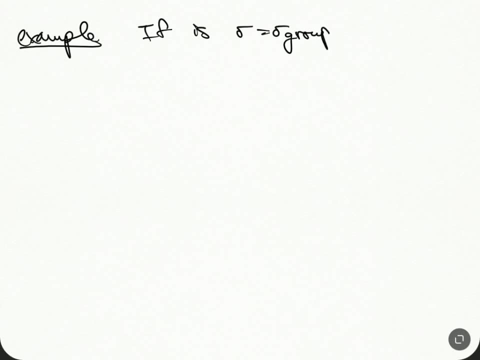 sigma group, then a sigma group structure is a set with you know a set, let's say S, with you know a multiplication operation, An inverse operation. so maybe we'll do it like this, So from S to S, and okay, and we 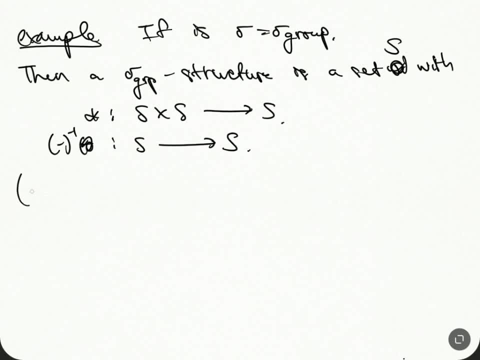 should note that that's it, that's all it is, and we should note that S, with these operations, does not necessarily satisfy the group axioms. okay, It's just something where you can formulate, where you can, you know, interpret the formulas. okay. 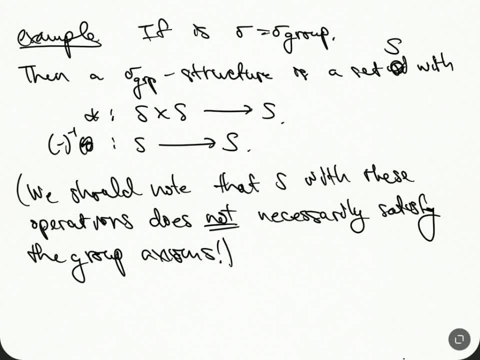 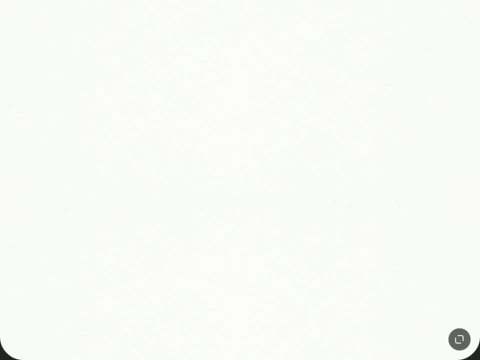 So that's it, So we can now give definitions. so theories: Maybe theories shouldn't quite go with semantics, but let's just give a definition. It's still a kind of syntactic thing, A theory, let's say four signature. 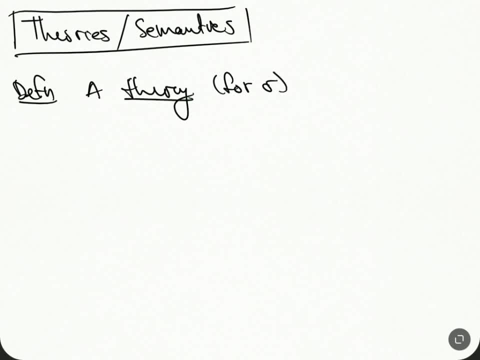 sigma is just a subset inside the language of four starter formulas. So these are. these are no free variables, Only integrals within a alphabet. Okay, so now I can define what a symbol means. so this really kind of a semantic thing. so 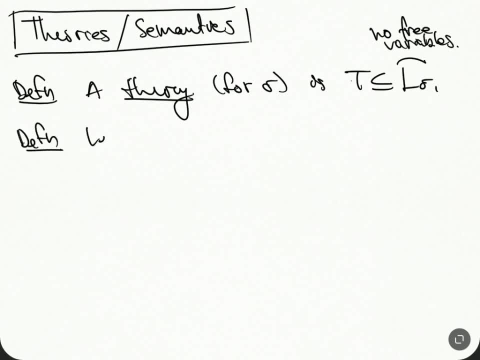 definitions: Let sigma be a signature. let phi be non-intuitive signature: Ok. TAG раза, a first order formula: okay. and so let M be a sigma structure: okay. so this thing, this is what we're going to define. we're going to define this symbol. M proves this. 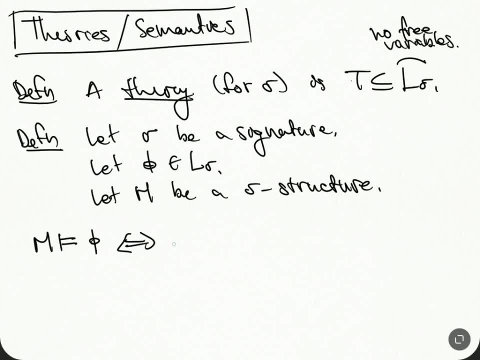 formula: phi if and only if. when we interpret phi in the structure M, it returns true, Okay. so sometimes we'll write true, it's like this, true, okay. and so we'll write a definition. M is a model of a theory, so this is M models: phi if and only if, so M. 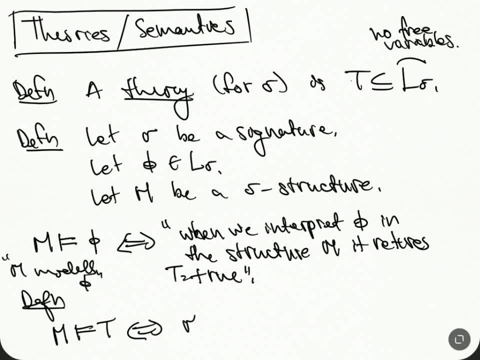 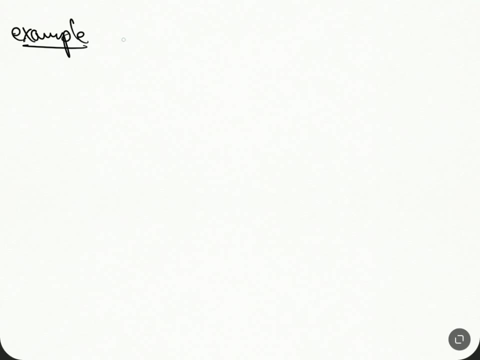 models phi if, and only if, M Proves, or M models phi for all phi and T. I shouldn't have said proved. there's a distinction between proved and being true. So the kind of the basic example is: if T is equal to the theory of groups, okay and so.